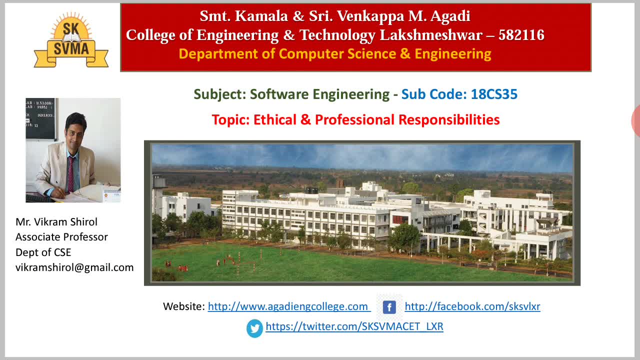 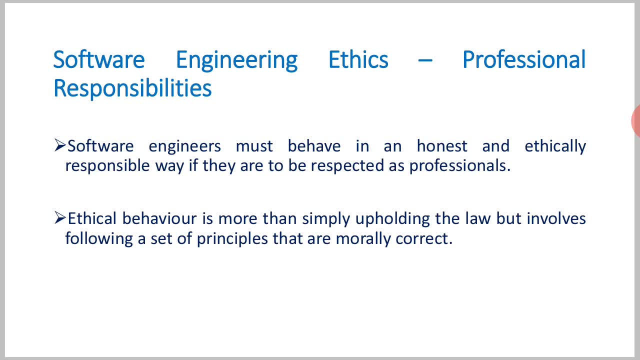 What are my responsibilities So that we are going to discuss in this particular video. So, basically, the software engineering ethics and professional responsibilities always deals with what The software engineering engineers must behave in an honest and ethically responsible way if they are to be respected as professionals. So we know that there are 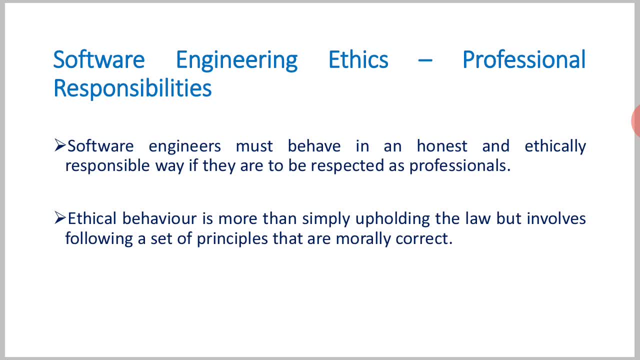 so many variety of professionals that are there in this society along with us. It may be a doctor, lawyers, Normally engineers, So within that, engineers. once again, we are mainly focusing on the software engineers because, we already told, software engineering is also one type of what. 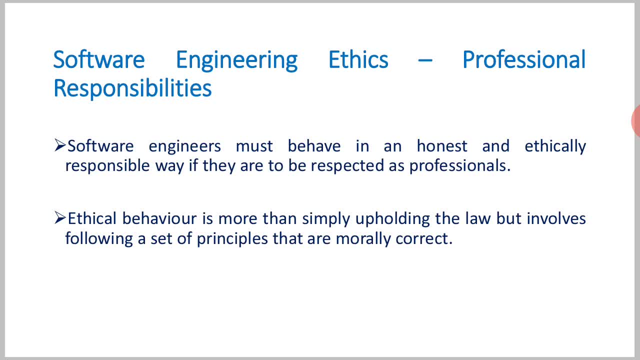 Engineering discipline, like mechanical engineering, like civil engineering. So software engineers should also. they have also, should they should also what Follow some sort of ethics and professional responsibilities. Okay, And in that this is a very important thing, is we need to behave as a honest and we should be ethically responsible. Then only the society. 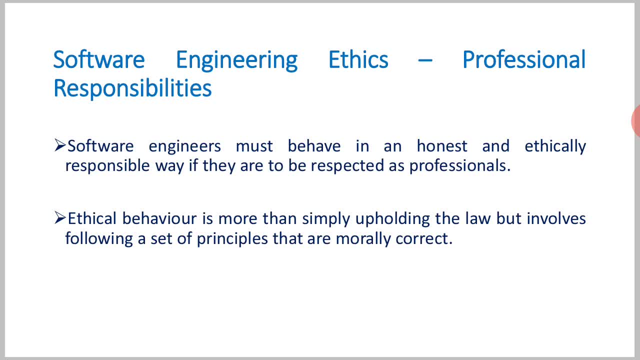 will give what A respect. Okay, So my colleagues will respect, or my employer will what Give respect. So that's very much essential. And another point is: ethical behavior is more than simply upholding the law, but involves what? Following a set of principles that are: 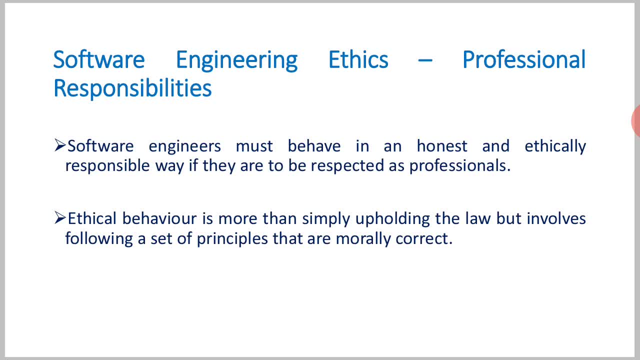 morally correct. That's very important, Okay. So never actually follow the law. That's very important. So never expect that you are going to behave as if some rules and regulations have been written on the paper. Okay, Always. ethics is beyond to that Ethics. 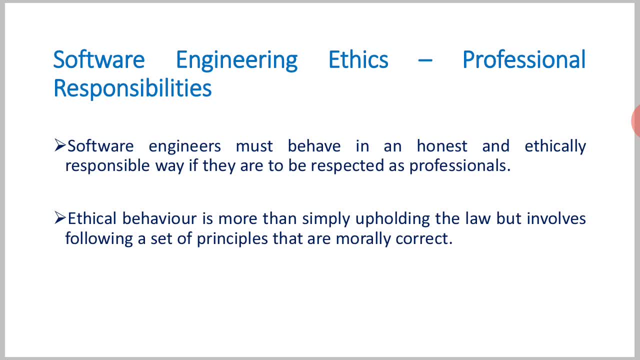 is what Always beyond to that, which is a set of what That are morally correct. Okay, So every time I need not to talk about only with respect to rules and regulations and laws, Okay, Apart from that being a human being. Okay, So we need to uphold the rules. 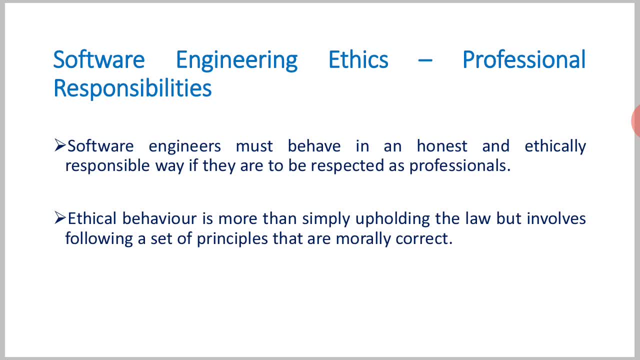 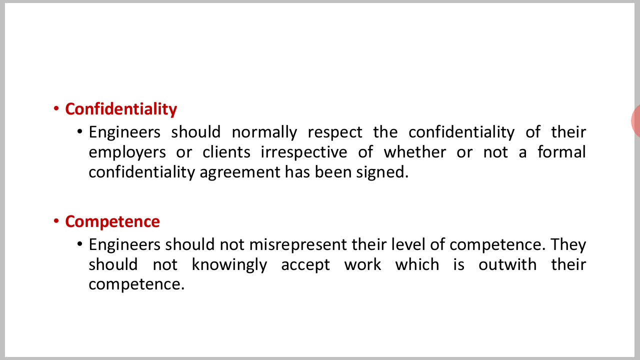 andäng uak, the universal human values that we need to inculcate, even though my profession is what? software engineering, or I'm a software engineer, So that matter Clear. So let's discuss with the responsibilities one by one here. The very first one is konfidentiality. 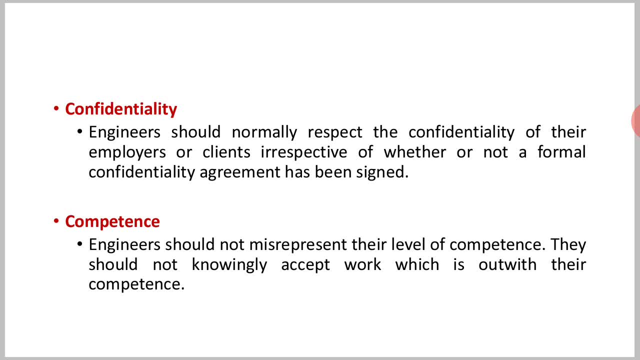 Okay, So being a software engineer, We have to maintain the confidentiality for whom we are working. 00 00 00 00.. means: 00 00 00 00 00 стен 00 00, 00 00 00 00ntит Señet. 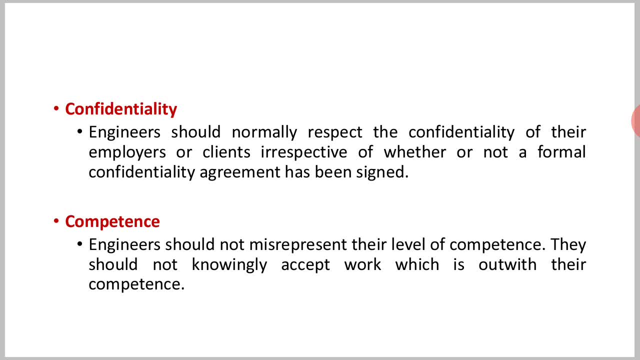 today, if I am working for one company, then it is my duty to maintain the confidentiality of what that particular organization. okay, as a software engineer, I might be working on some particular project, so I should not disclose that. I should not disclose to some third party. I should not misuse. 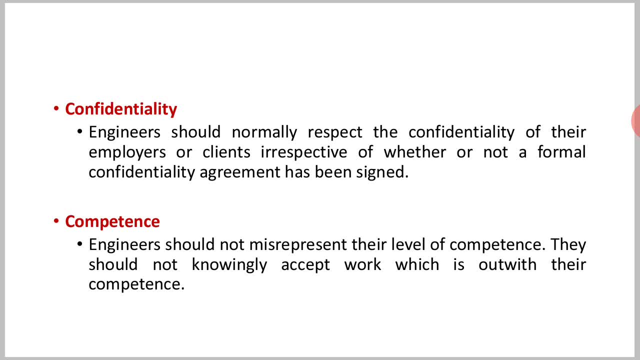 that. or even if I am working for some particular client, if I am developing some software for some client, okay, the same information should not be get leaked by me. that care should be always what taken, so like that, in every profession they are having, the confidentiality matters will be there. 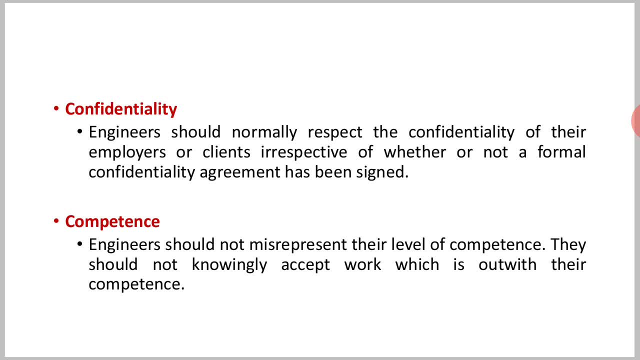 even in medical. in medical field also, okay, the patient information should be always what confidential. so it's the job of the doctor that he has to maintain that. similarly, being a software engineer, it is my responsibility to maintain the confidentiality with respect to what my organization where I am going to work. okay, that's the very the first point. 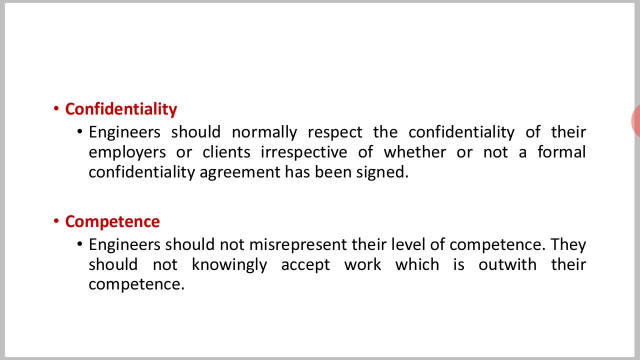 for what? the professional and ethical responsibility. second one is a competency. it's a competence. competence means what? so here, as a software engineer, I should not misinterpret myself, my or my level of competence. see, for example, say I am working in some company as a software engineer, my senior. 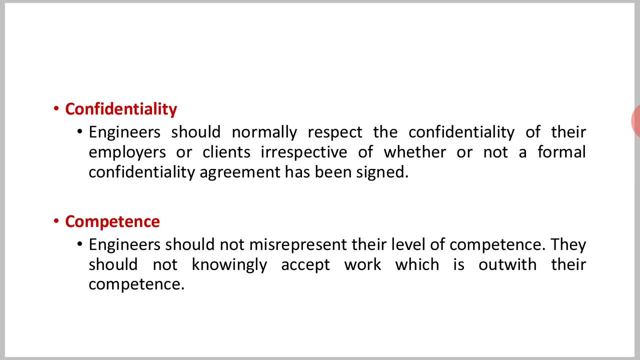 or one of the project manager will come to me, either clear, and he will say that, okay, one extra work is there, I am going to hand over it to you and I will give you one week time and you can please finish it off and simply if I say, yes, sir, I can do it, but later after one week, okay, if I can't do that. 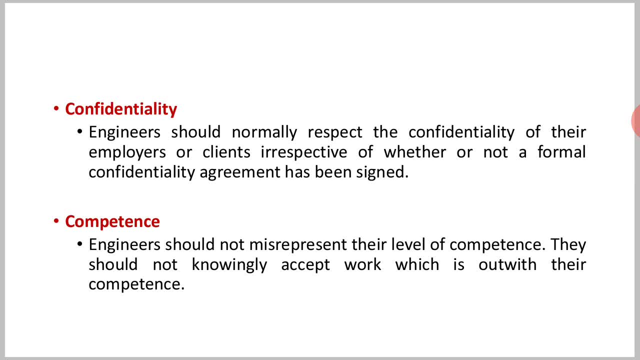 because I will be knowing that the task given to me is impossible from me. I, because I may not be expert in that particular technology. okay, when I know that I cannot be expert in that particular technology. okay, when I know that I cannot do that, honestly, we should accept that. yes. okay, we would have told that to the 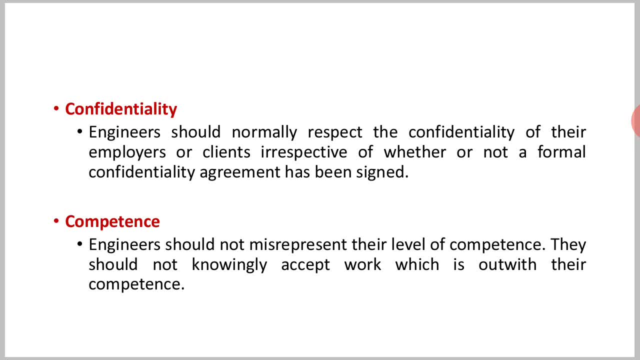 manager saying that: no, sir, I don't know that. at least we can save that one week time. okay, so you should not misinterpret anyone okay in the organization. saying that, what if I don't know that particular work? honestly, I need to accept. saying that it is beyond to me, I cannot do that. okay, so that is what. 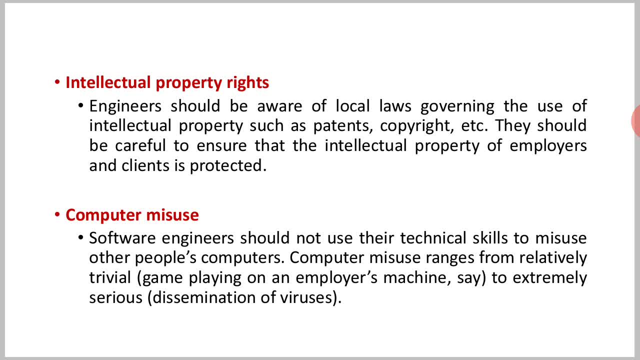 competence. then the third one is: intellectual property rights is very important. okay, so every software engineer should be abide by rules and regulations and laws of defined by either it may be a government, okay, how it may be the I PRS, like intellectual property rights, such as what the patents copyright? okay, that we need to follow others and even I need to. 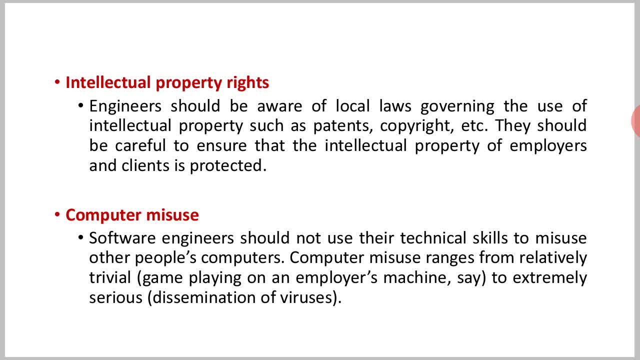 follow the rules and regulations and loss defined by what my own organization, where I am working, I cannot break those rules and laws only by 쓸 이�palis lyrics is most important when you are dealing with soft Chairman financial property- okay, I am working, I cannot break those rules. Sean is responsible for communication contracts to the end vision process, advance funds, та aircraft and the role part that I need to mark phonGS. so far, that is quitefluous. 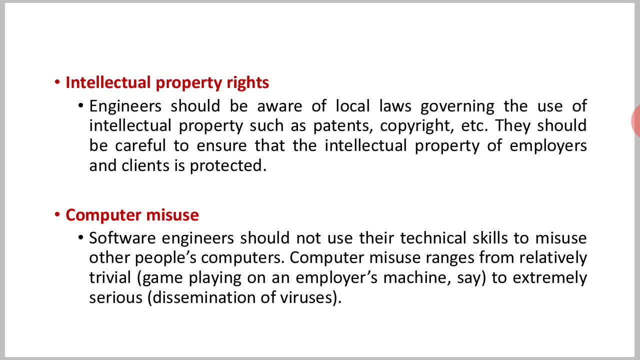 okay. so, even being a student, I am not supposed to take the rough copy of one textbook which is having a copyright. it's wrong, actually. okay. so, being a software engineer, I should not misuse the software's which belongs to my company and to install in my own PC for my personal purpose. that should not. 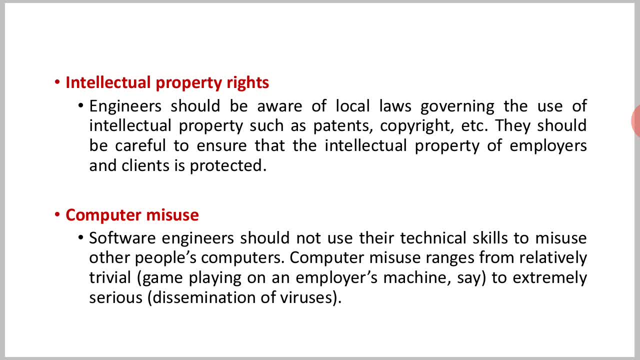 happen. okay, I should not do such kind of what piracy things that is not happen. then the last one is: what computer misuse? okay. so being a software engineer, even here the suggestion is okay, not to use our technical skills to misuse what the others- computers or laptops, whatever it may be. okay, even it. 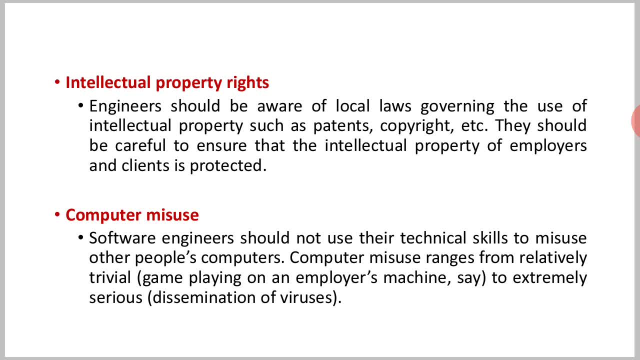 may include the beginning level, that is, from what you call playing a game on an employer's machine is also what wrong without the permission, even though I am close with my subordinate, without the permission of that my colleague, I am not supposed to sit on his seat and use his.